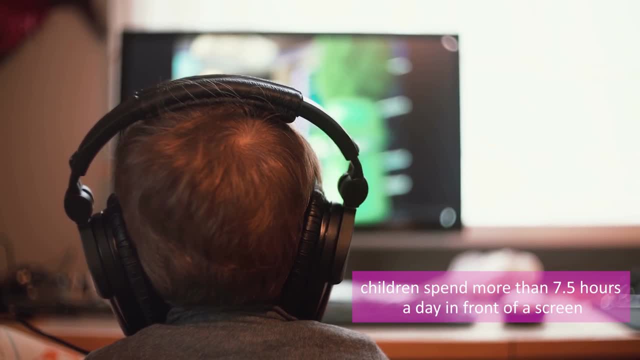 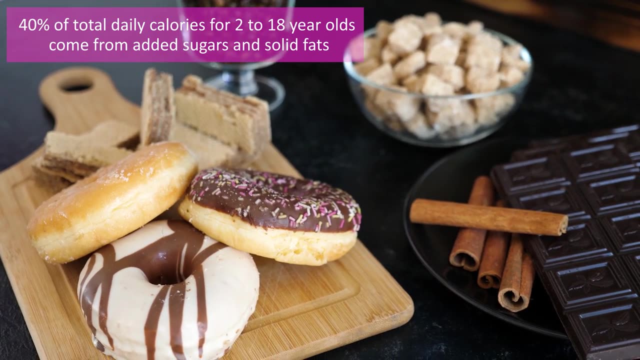 each day. Children spend more than seven and a half hours a day in front of a screen And for two to 18 year olds, 40 percent of their total daily calories come from added sugars and solid fats. All of these numbers come from data and statistical analysis of this data. 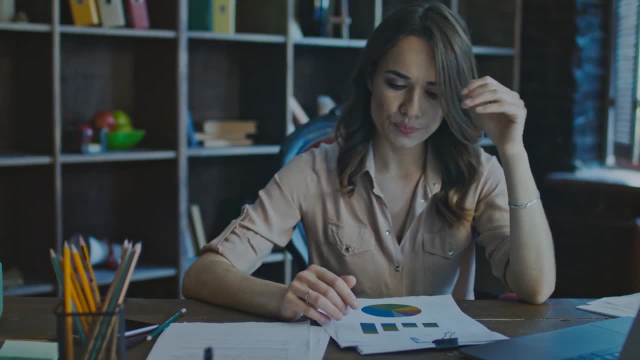 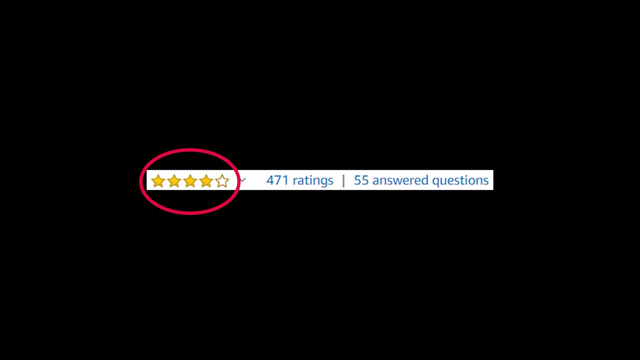 And what statistics actually does is gives us people a way to make informed decisions. For example, if you've ever bought something on Amazon, you probably look at the star ratings If you find two similar versions of a product you want, say a camera lens. 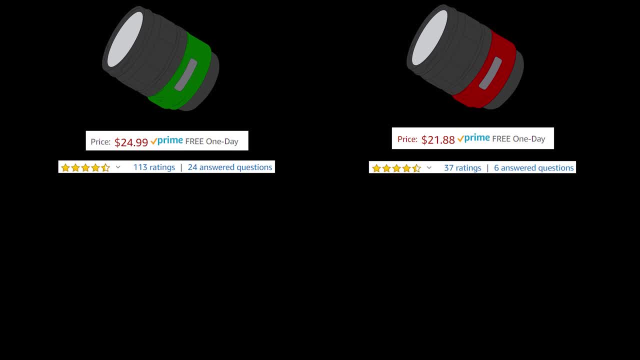 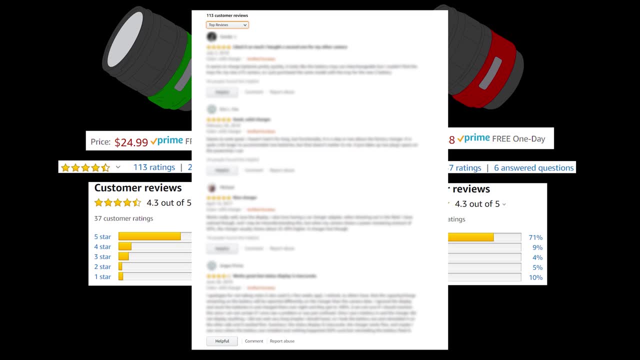 you look at the price of each, then how many overall stars it has, then maybe the distribution of the ratings and how many total ratings it has, and maybe read a few of the highest and lowest reviews about the lens. Then you're going to look at the sellers of the lens and check out. 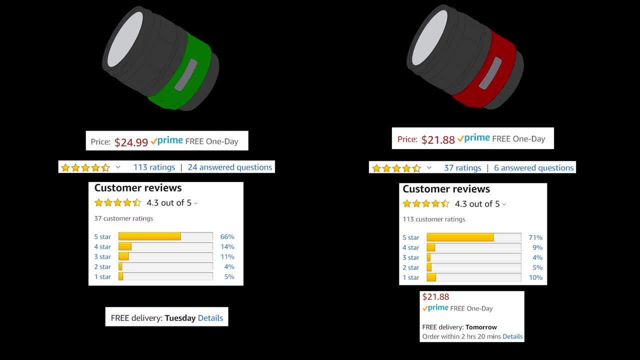 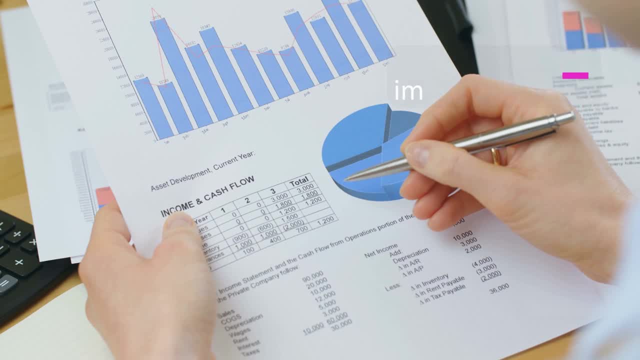 their ratings and then you check out the delivery time until you have the product in your hands. In this scenario, you would have done a very quick and informal statistical analysis. In learning about statistics, there are some important terms to have a basic understanding of. 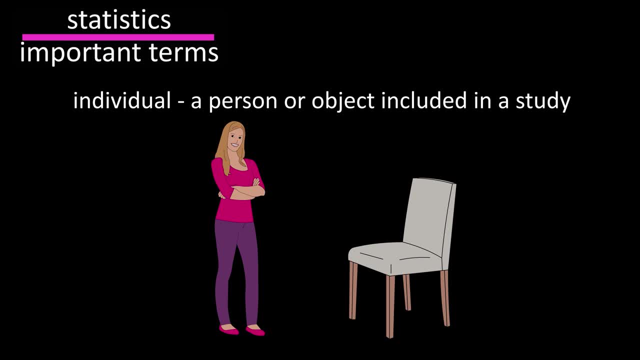 An individual, also called an element, is a person or object included in a study. Variable is characteristic of the individual being measured or observed, which varies from individual to individual. Variable is characteristic of the individual being measured or observed, which varies from individual to individual. 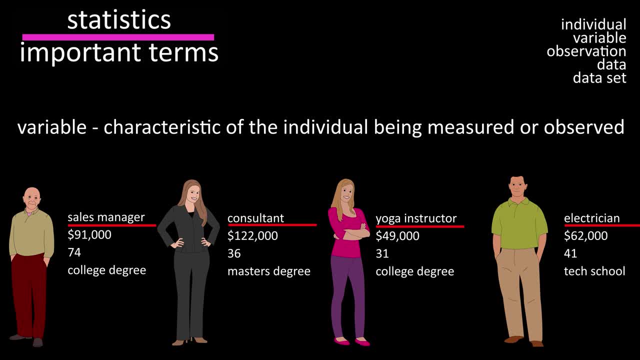 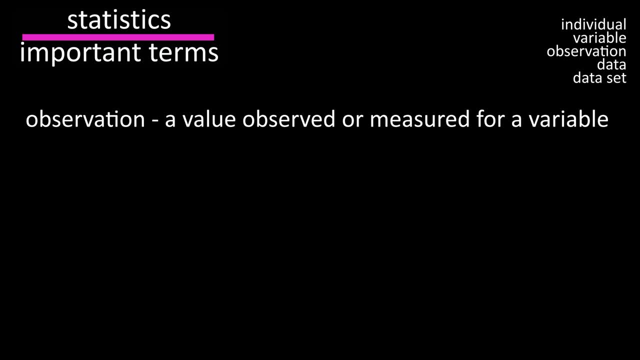 Variable is characteristic of the individual being measured or observed, which varies from individual to individual. So, for instance, this could be occupation, income, age or education. Observation is a value that is observed for a variable, which is also called a measurement. 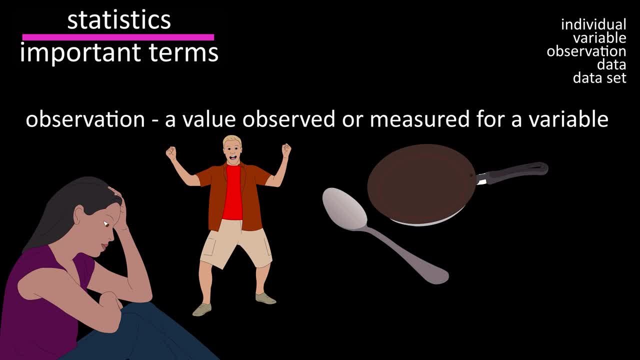 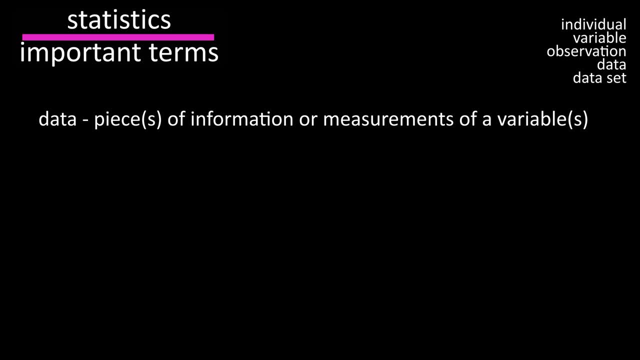 and a person can actually be an observation, as can a certain product or even a set period in time. Data is a piece of information, or pieces of information or the values or measurements of a variable collected on individuals. All of these would be observations for each of the different variables. 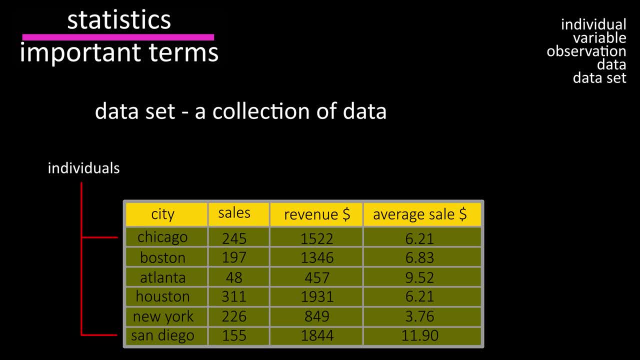 Data set is a collection of data, so this table lists the individuals, the variables and each of the observations for each of the individuals. This little table here would be considered a data set. My friends, this is the first video in a series of videos I'll be posting about understanding. 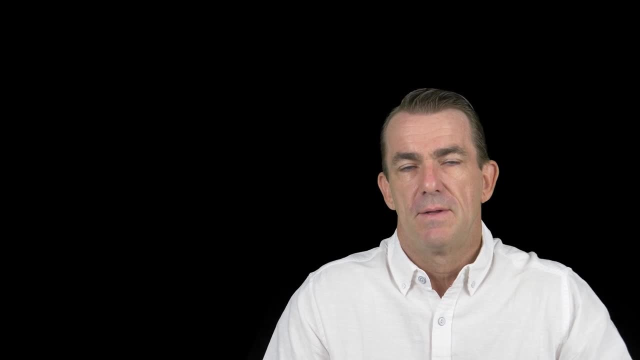 statistics. I've got more videos right there for you Till next time I am outta here.